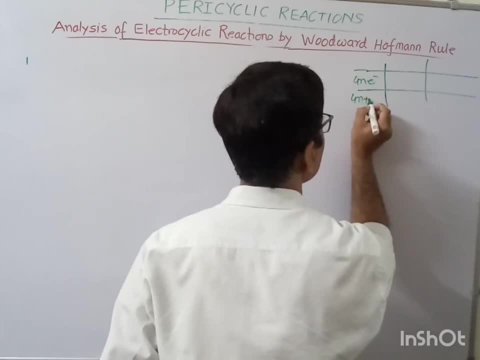 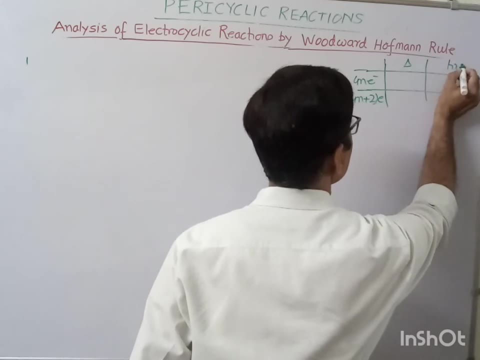 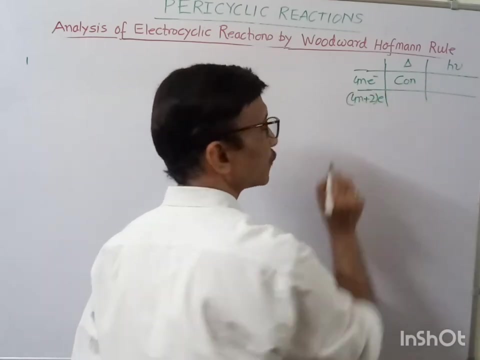 4N electron systems and we read for 4N plus 2 electron system. So 4N plus 2 electron systems can be analyzed under thermal condition or under photochemical condition. Under thermal condition, the end orbitals will undergo on rotation. in case of 4N electron system, 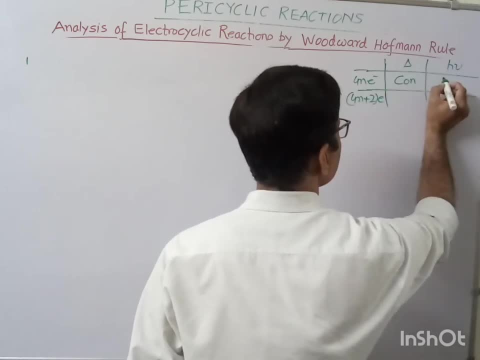 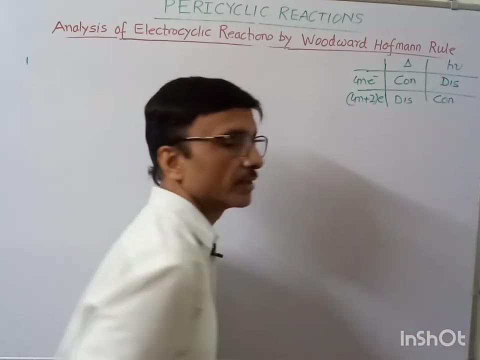 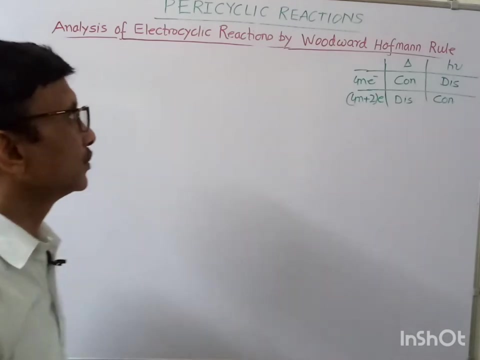 and under photochemical systems these orbitals undergo dysfunction, and opposite is the case for 4N plus 2 electron system. okay, So this rule we have to analyze with the help of Woodward Hoffman rule. So according to this way of elimination, we can analyze the electrocyclic reactions by the 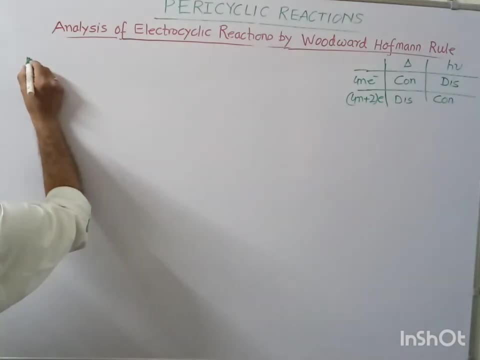 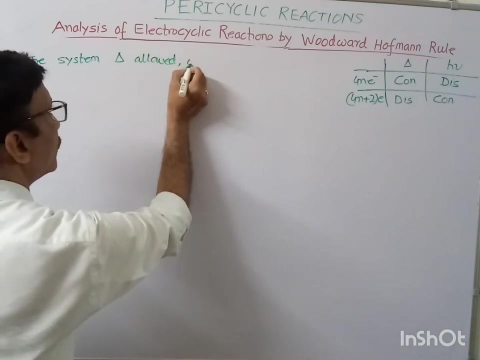 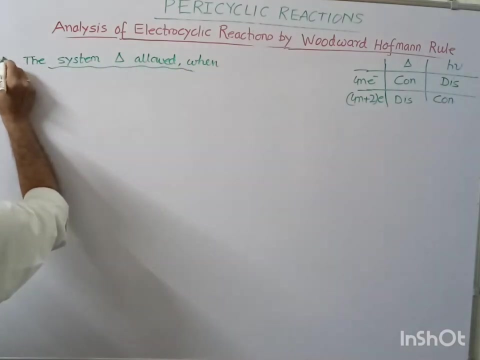 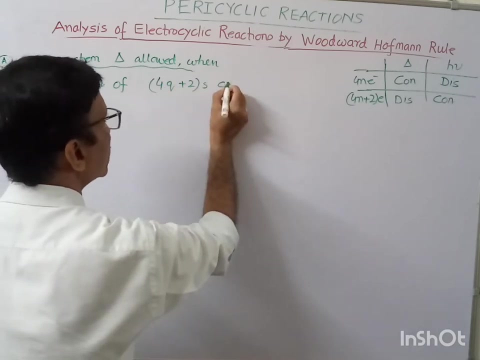 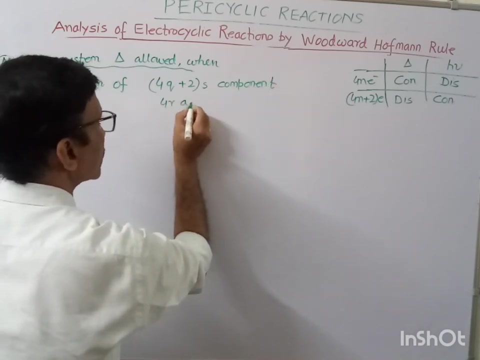 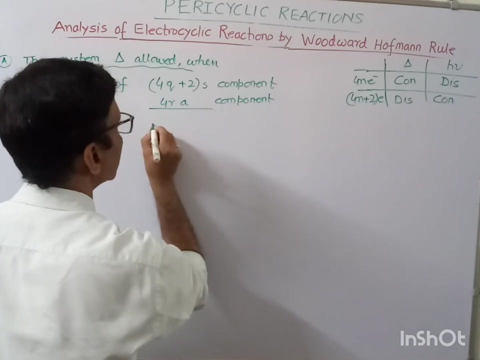 Woodward-Hoffmann rule: if system is thermally allowed, the system is thermally allowed in in what case? the system is thermally allowed when? this is when the sum of 4Q plus 2S component and 4R component is coming out to be odd. 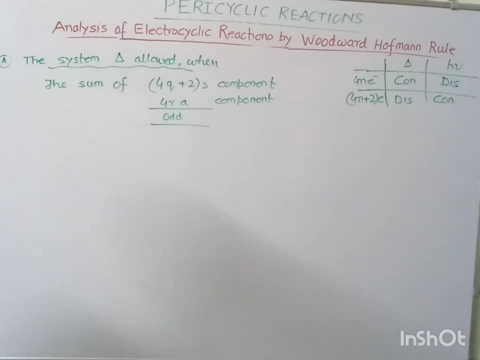 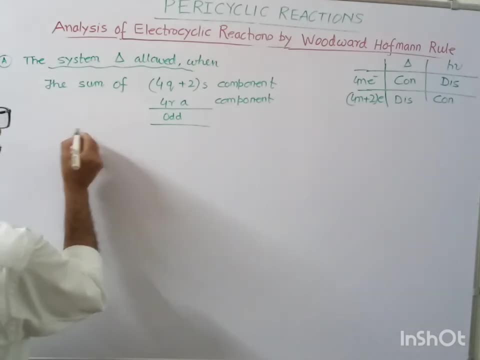 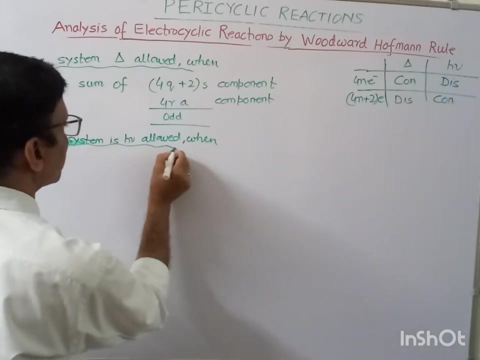 you now suppose, if sum of you now suppose, if sum of second case, suppose the system is photochemically allowed, then the sum of photochemically allowed, then the sum of photochemically allowed, then the sum of true is phot��ung food plus three so-called true is phot 발, true is phot komma. hice antenna to add to a photochemical out, when the sum of two nibex will be allowed to be allowed to be connected into a photochemical out, when the sum of three, with four q addition to e plus a. 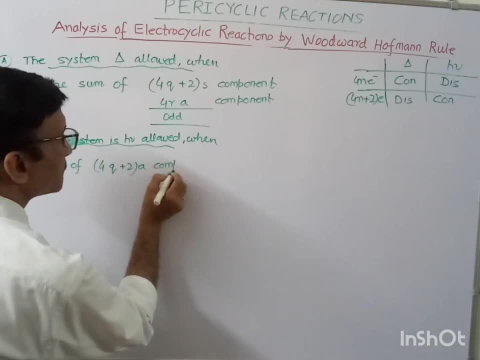 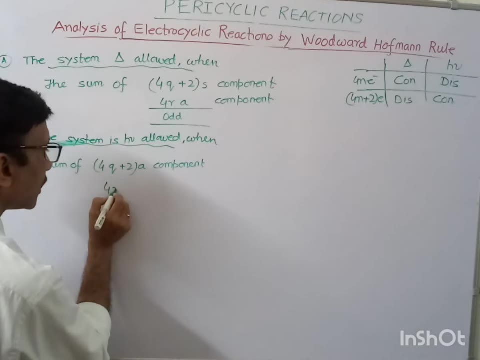 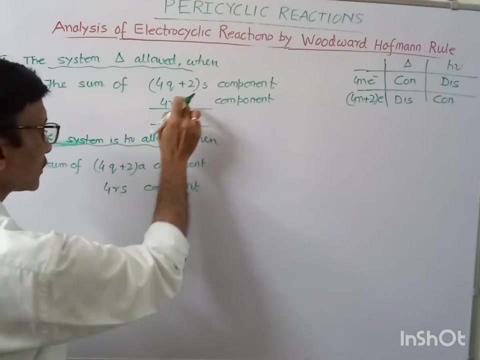 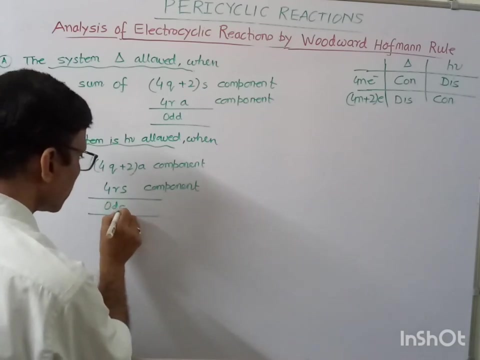 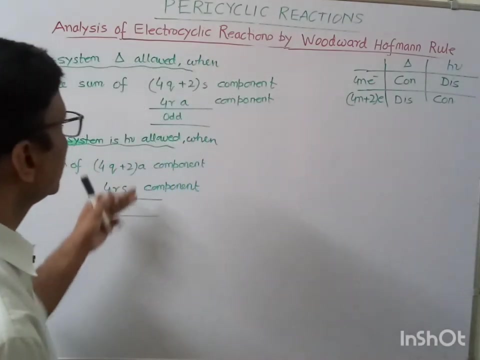 two: A component- here in place of S- now I have written A. and four are S component in place of A- here I have written S. So if some of these two component is coming out to be odd, then our system is photochemically allowed. So let us see the meaning of here: Q or R, S or A. 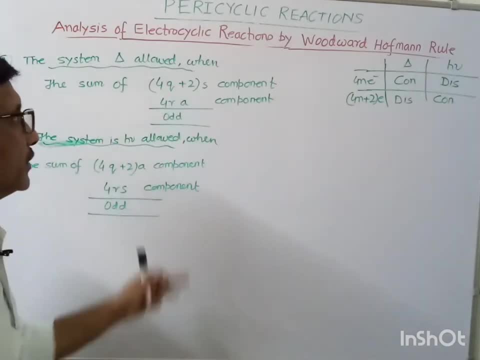 Now suppose two type of system, either 4Q plus 2 system or the system may be 4R system. So when we say the system is 4Q plus 2 system, So suppose, if, if, if I put 4Q plus 2, this is equal to number of pi electrons. Suppose, if we put 4Q plus 2 is equal 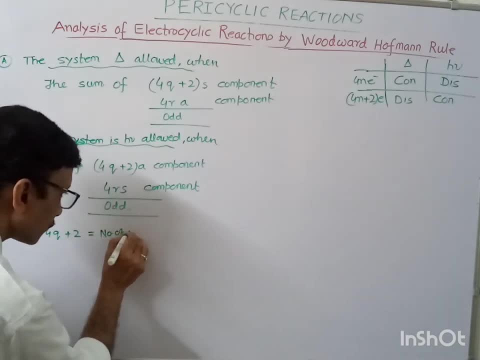 to number of pi electron, number of pi electrons. and suppose: if we get, if we get we get, Q is equal to 1, 2, 3, like this: Then system is odd, zero. We can say 0, 0, 1, 2, 3.. Then system is 4Q plus system. 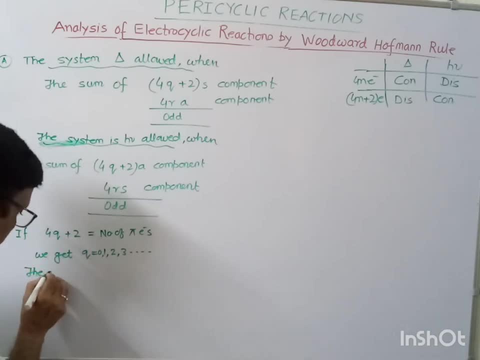 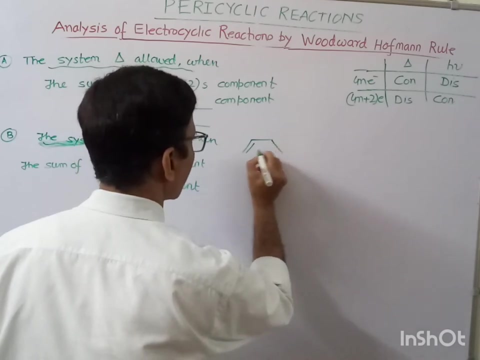 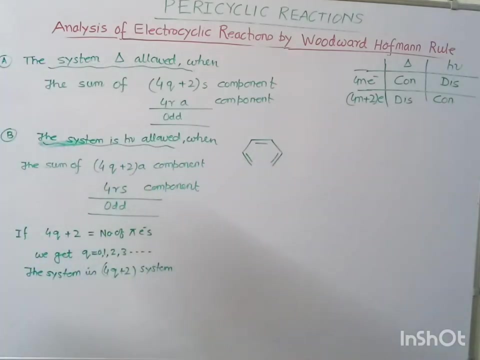 4Q plus 2 system, Then system is 4Q plus 2 system. So this is one of the case. So I will make a suppose. Suppose I take this butadiene, or suppose I take hexatrine, and in hexatrine suppose I put 4Q plus 2, equal to number of pi electron. 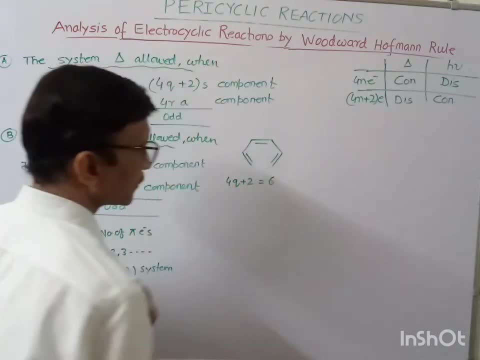 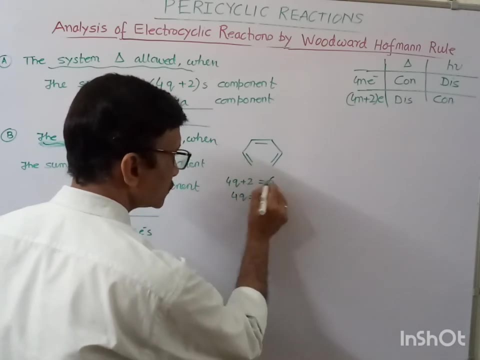 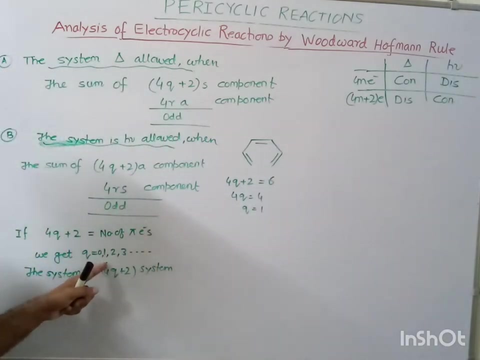 So number of pi electron here is 6 and here Q is equal to now. if you will see 4Q, this is equal to 6 minus 2, that is equal to 4, and Q is coming out to be 1.. So here Q is coming out to be 1.. So that is why such system may be called as 4Q plus 2 system. 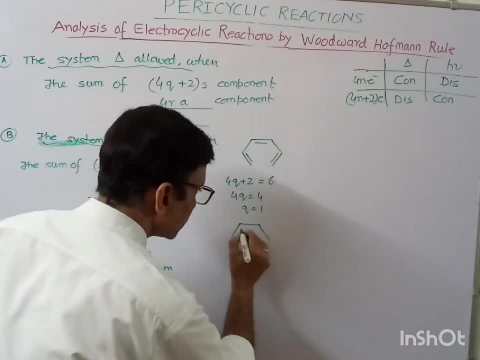 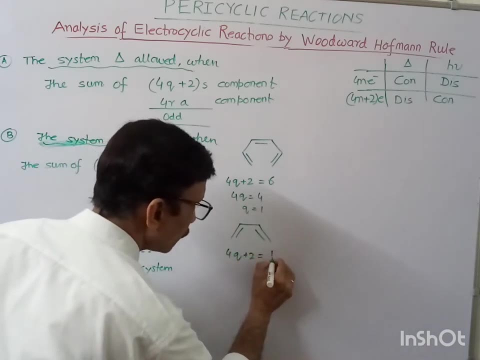 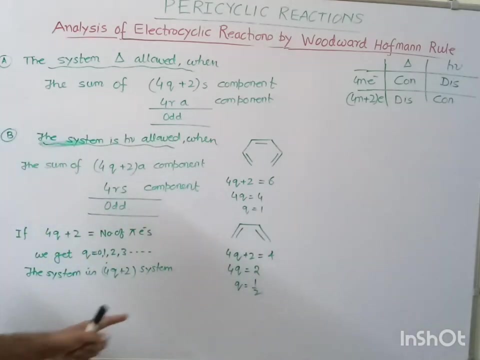 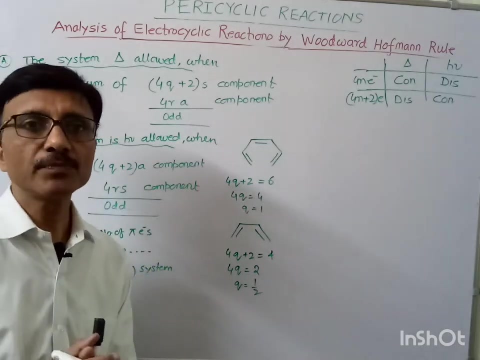 Now suppose I take butadiene, this system, and if you put hexatrine, 4Q plus 2, this is equal to 4. here, how many pi electrons are present? number of pi electrons: 4.. Then here Q is not coming out to be, here 4Q, this comes out to be 2, and it is equal to 1 by 2.. So Q is not coming out to be either 0, 1, 2, 3.. So that is why such system can't be called as the 4Q plus 2 system. 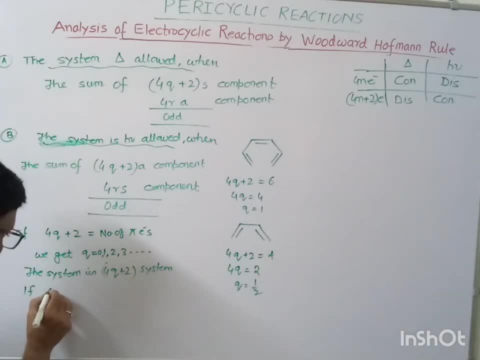 Now next thing: if, If 4R, suppose if 4R, so 2 type 1 is 4Q plus 2 or 4R or 4R. So if 4R is equal to number of pi electron, if we put, if we put 4R is equal to number of pi electrons, and we get: Q is equal to 0,, 1,, 2,, 3.. 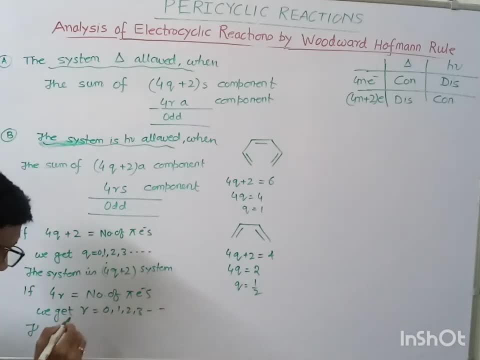 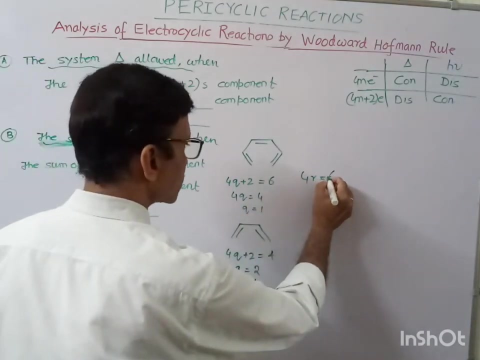 Then system is called as: so sorry, then if we get R is equal to 0,, 1,, 2,, 3, then system is 4R system. Now let us see here: put 4R. if we put 4R is equal to number of pi electrons. so number of pi electron is 6.. 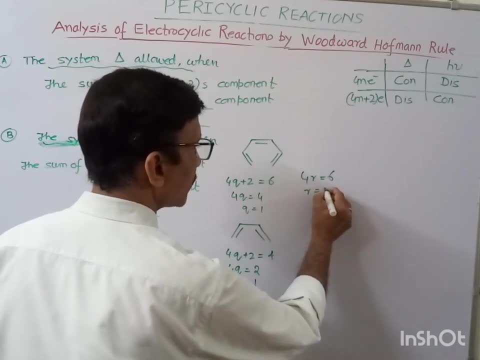 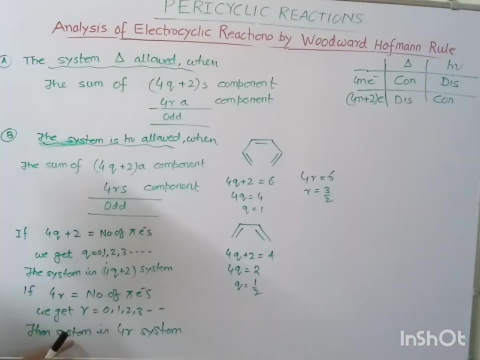 So R, we will get how many. what is the value of R? it is 3 by 2.. So R is not equal to 0,, 1,, 2,, 3. that is why it is not. it is not 4R system. 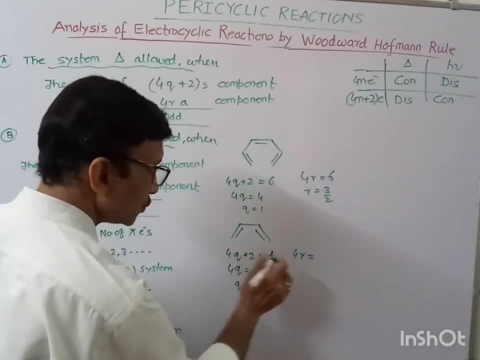 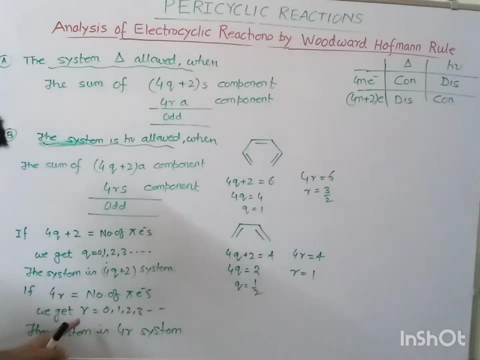 Now, if you here, if you will see if 4R is equal to suppose I put 4 number of pi electron, here is 4 and here we are getting R is equal to 1.. So here we are getting R is equal to 1. that is why it is 4R system. 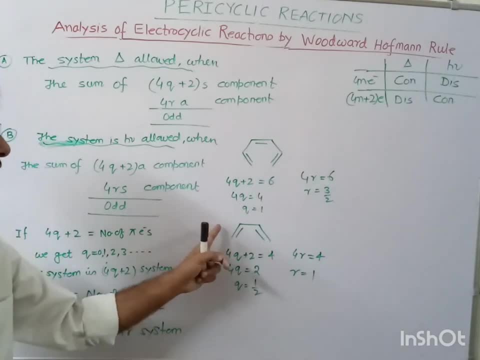 In a same way, suppose, if we take, if we will take the this one, So this is 4R, So this is 4R, So this is 4R material, so this is total R, R1, 4R. 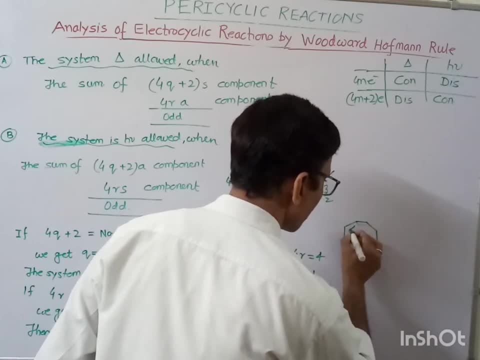 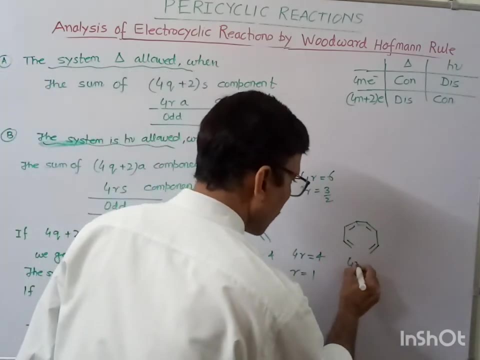 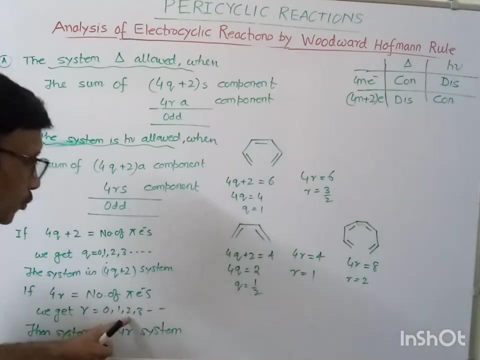 So now, if you look here in octatetrine data train, suppose the 4 R this is: this- comes out to be 8. So this R D C is equal to 2. So R is coming out to be two. that is why this is our 4R system. 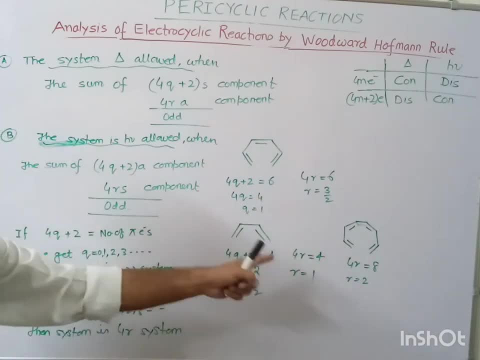 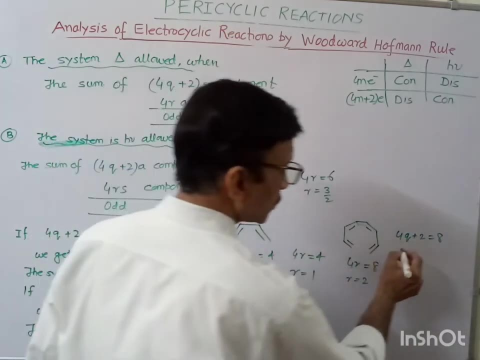 And here this R Q will not come out to be. in this case, suppose I put 4 Q D, where Q, q plus 2 is equal to 8. So this q 4q, this is equal to 6 and q comes out to be 3 by 2.. 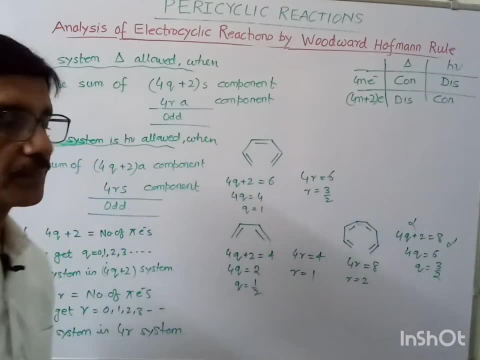 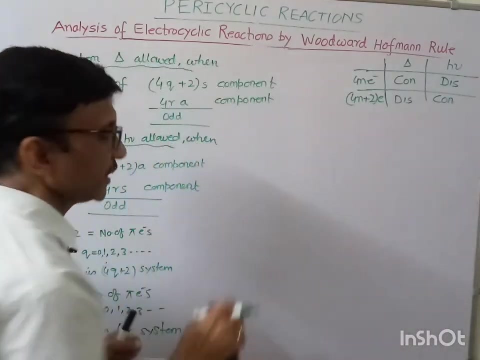 So that is why it is not 4q plus 2 system. So like this, we may understand for this. what is this 4q plus 2 or 4r system? Now let us see what about this. what is the meaning of this a and s? what is the meaning of this a and s Now, this a and this s. 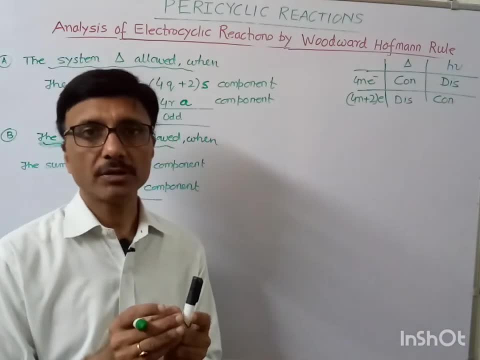 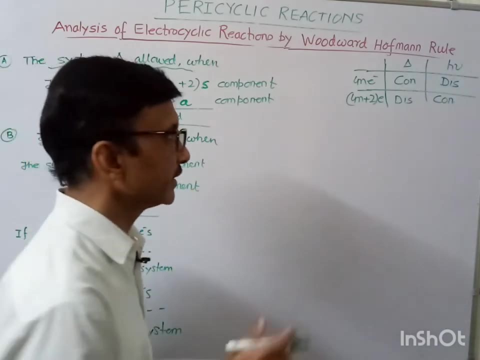 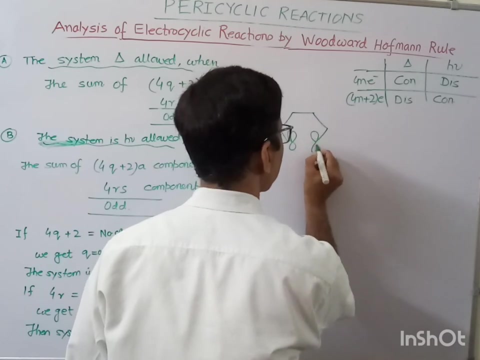 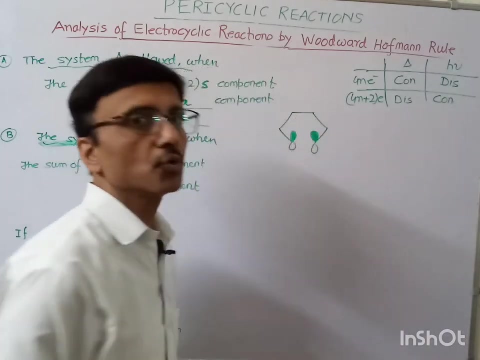 s means when the, when the antelope, when the antelope which combines to form a bond is on the upper side. Suppose this is okay. this suppose for the bond formation if two upper lobes, both upper lobes, involved in the bond formation. 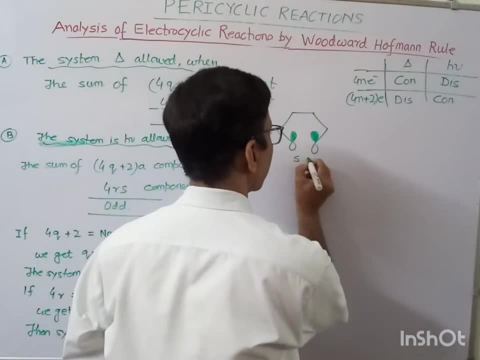 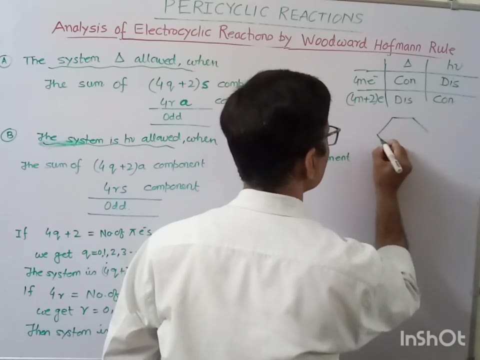 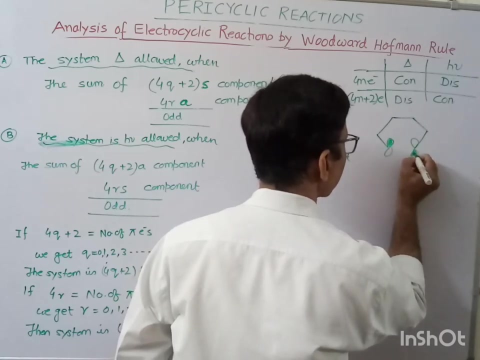 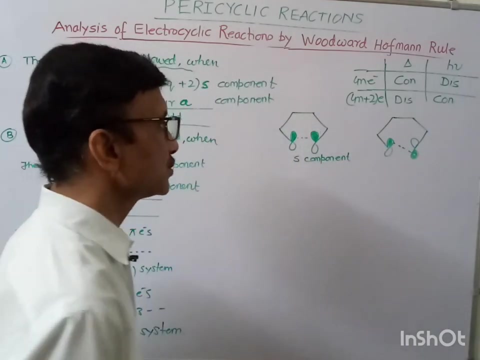 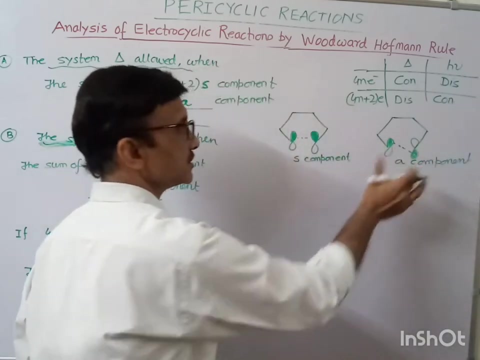 then such is. it is called as the s component. It is s component, And for bond formation, suppose one upper and one lower lobe is involved, one upper and one lower lobe is involved in one formation, Then such system is called as the a component. Or we may also see: suppose this is supra and this is entra. 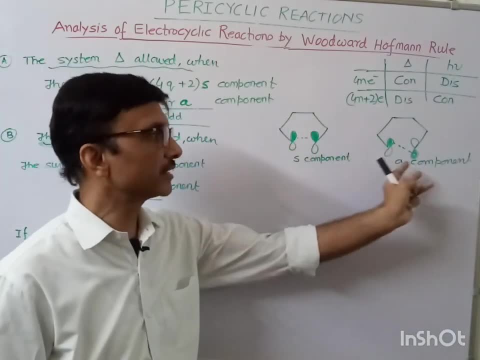 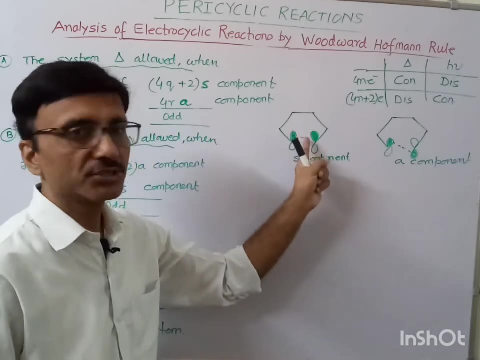 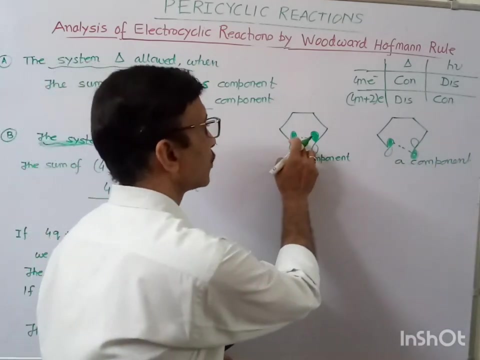 we may also call it work, But so this is s component and this is a component. So either we know that the bond, the bond formation may occur via this rotation, and here the bond formation may occur via the con rotation, No doubt this bond will form. 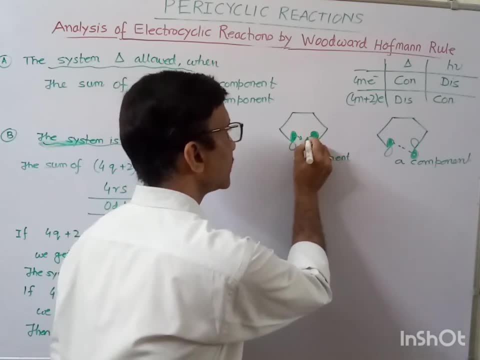 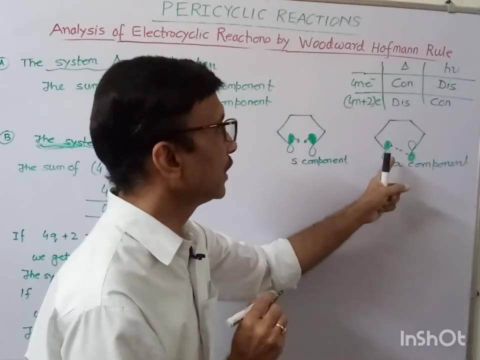 when it will form, When the both orbital will move in opposite direction. Okay, So it means when both orbital move in opposite direction, it is s component. If it is moving in a the same direction, both orbitals are moving in the same direction. 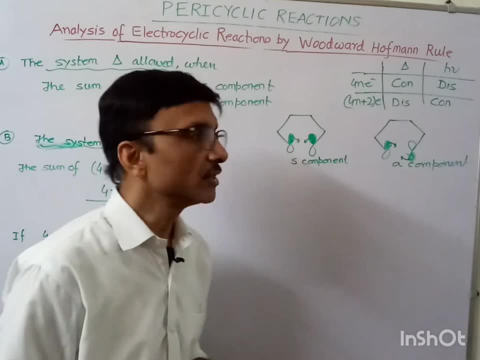 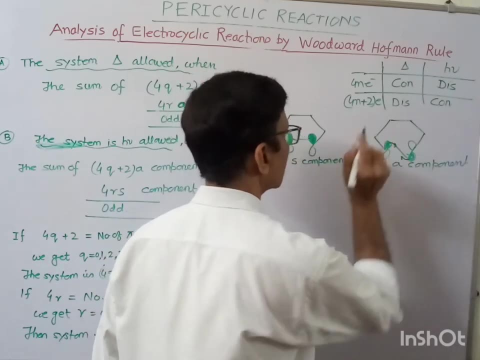 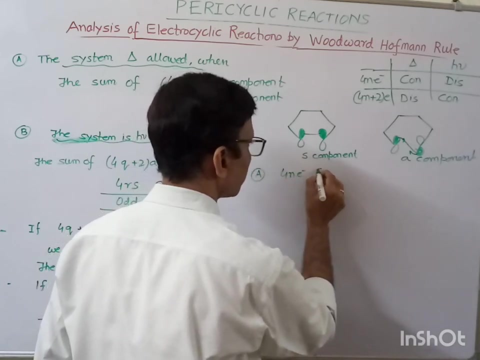 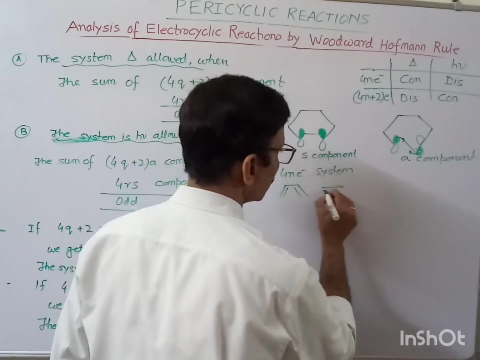 then only these two opposite lobes may combine. So this is the bond rotation. So this is the thing. okay For this. first for an electron system, For example, If suppose butadiene, it converts up into the cyclobutene. 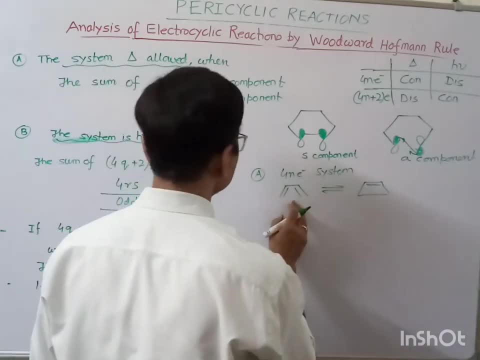 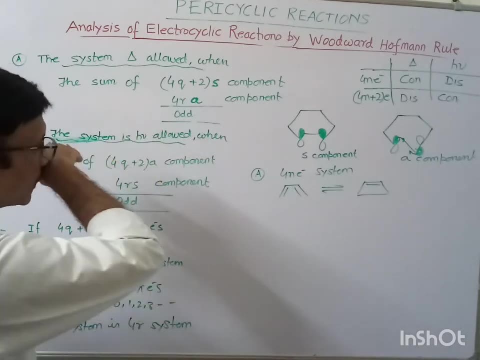 Okay Now. So this is our, this is our. what kind of system this is, what kind of component we can see? This is 4R. this is our 4R. This is 4R. Why It is 4R. 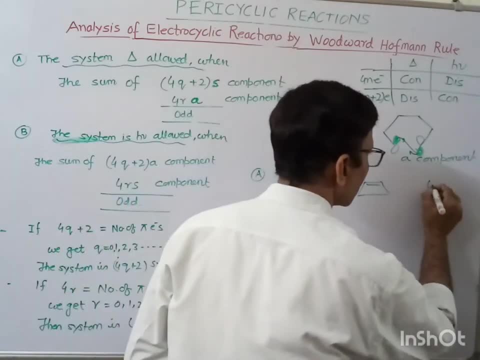 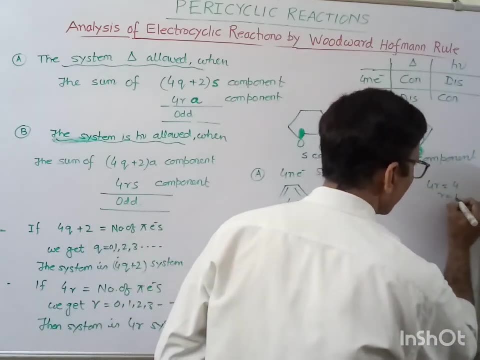 Why It is 4R. because this 4R, if we put 4R, is equal to how many pi electrons this comes out to be. this is 4,, so R is coming out to be 1.. So if R is coming out to be either 0,, 1,, 2,, 3,, then such system is 4R system. so this: 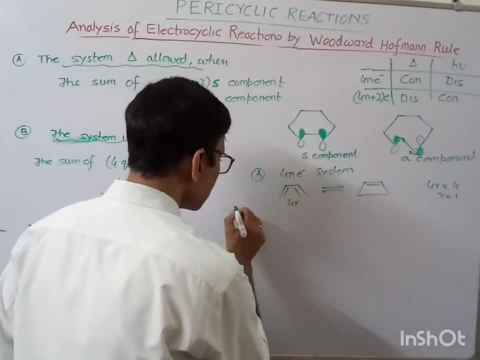 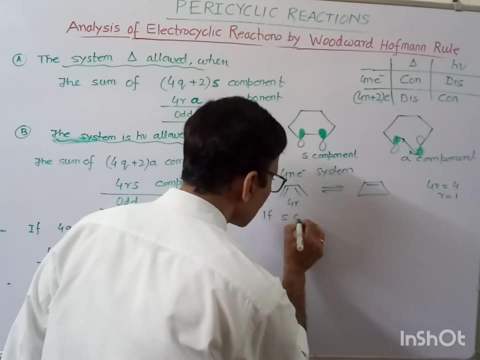 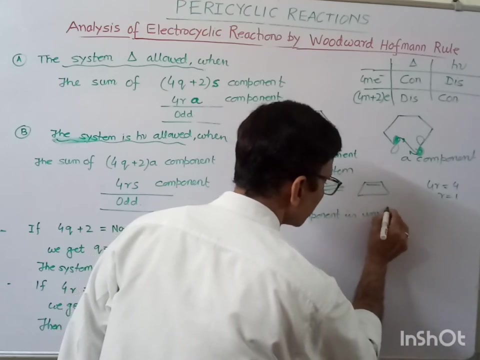 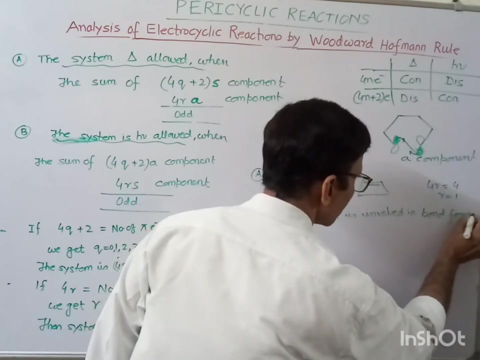 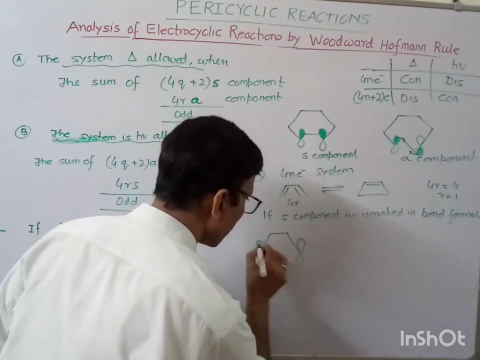 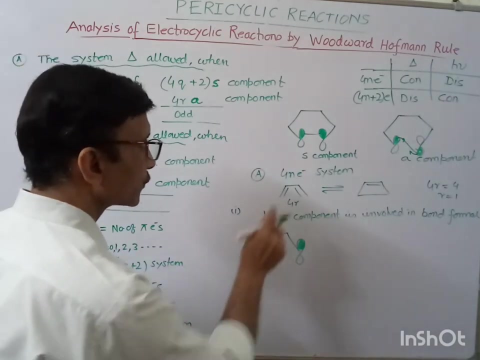 is 4R system. Now let us take two case. first, suppose if S component is involved in bond formation. if S component is involved in bond formation, it means S component means both upper lobe is involved in bond formation, both upper lobe is involved in bond formation. this is: 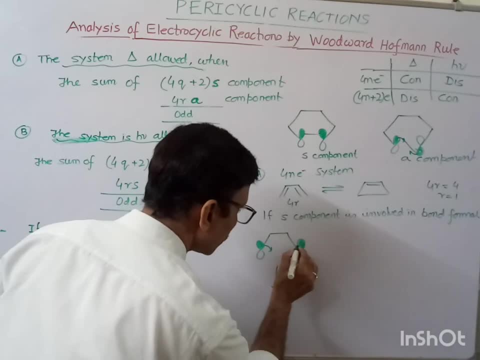 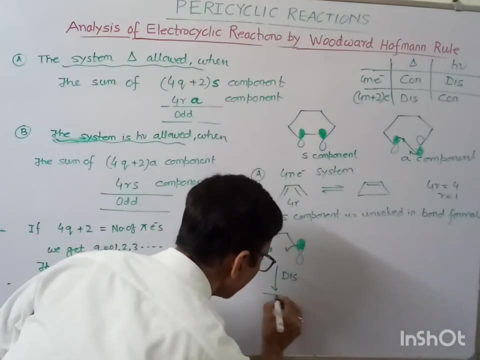 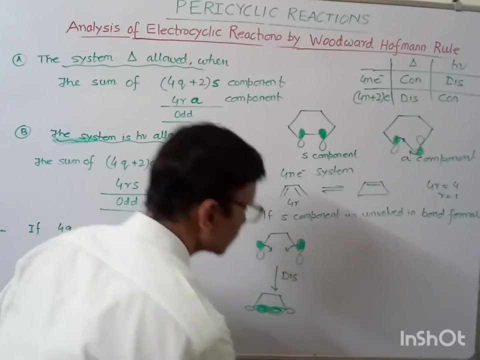 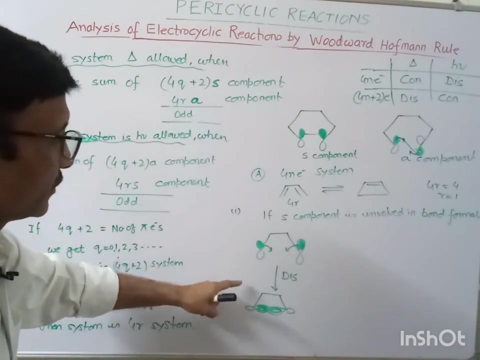 S component, then it may undergo bond formation when this rotation of orbital takes place. Now you will get the bond, you will get the our product, that is, you will get this product. Now suppose we have to check whether this condition is allowed thermally or photochemically. 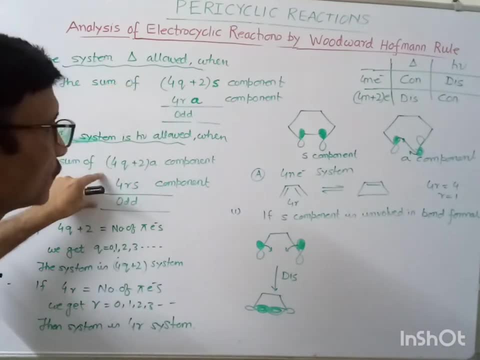 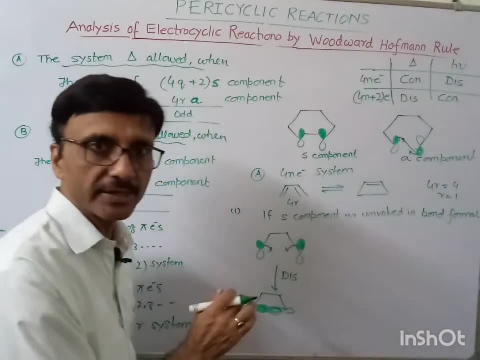 for this we have to check. Now suppose we have to check whether this condition is allowed thermally or photochemically. we have to see the sum of these two, or we have to see the sum of these two. Now, here this is our 4R, and when S component is involved, then it is 4RS. you see, overall, 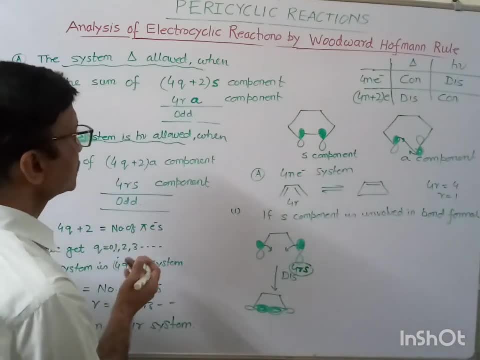 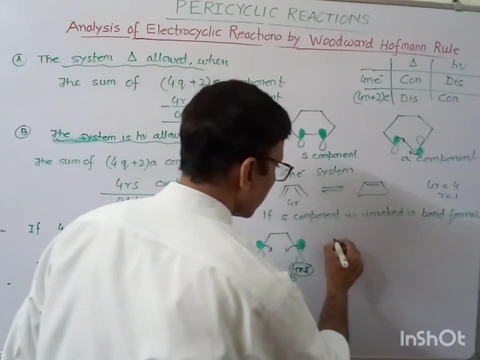 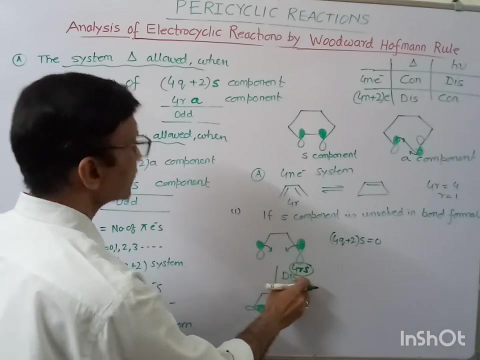 this is 4RS component. It means all this 4Q plus 2 system. 4Q plus 2S is 0, so that is why we can write: 4Q plus 2S is here 0, because this is 4rs. In the same way, 4ra, 4ra is also 0, so it's. 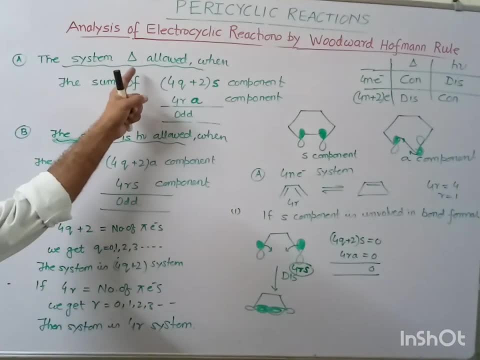 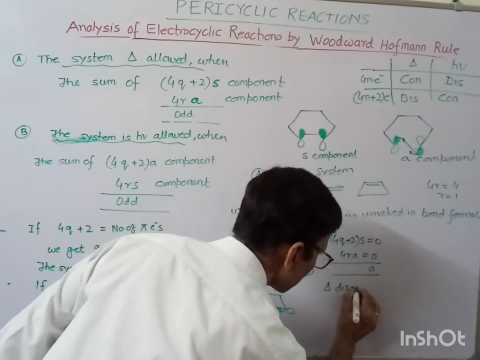 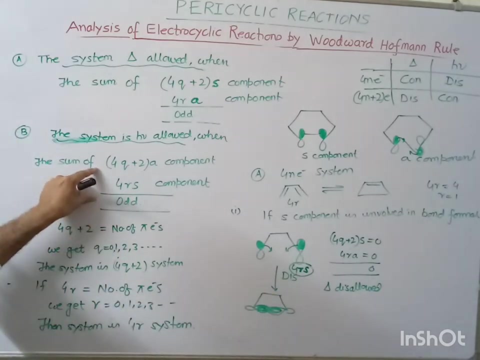 come out to be 0. So, therefore, this is: it is not coming out to be odd, so that's why it is thermally disallowed, thermally disallowed, So this rotation here is thermally disallowed. Now we should check for whether it is photochemically. 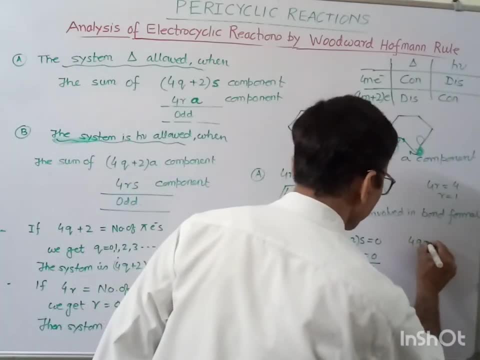 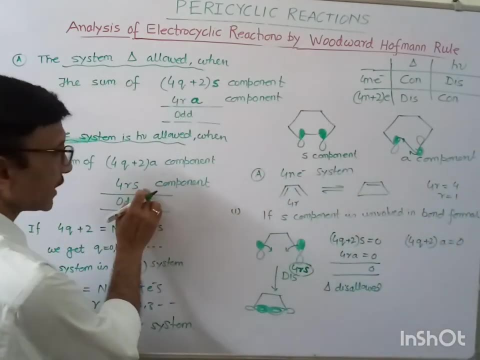 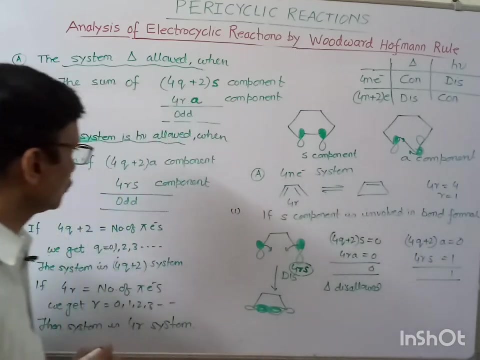 disallowed. So here, 4q plus 2a, this is also 0, this is also 0, but 4rs is 4rs is 1, 4rs is 1.. That's why it is coming out to be odd this is. 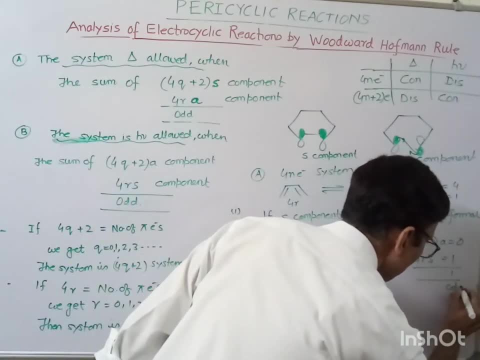 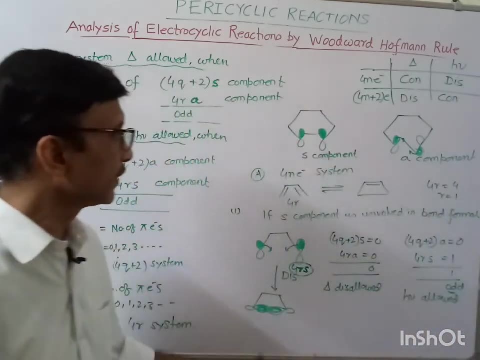 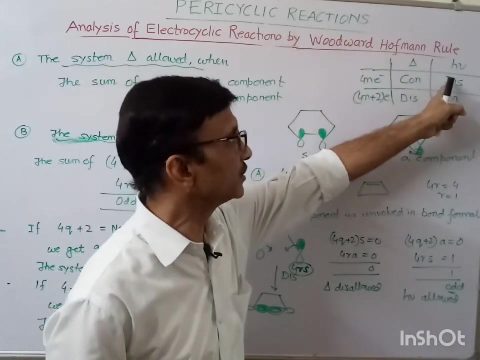 coming out to be odd. this is odd number. that's why it is photochemically allowed. It is photochemically allowed. So same thing you can say like see for Fourier electron system: when this rotation occurs, it means it occurs only under. 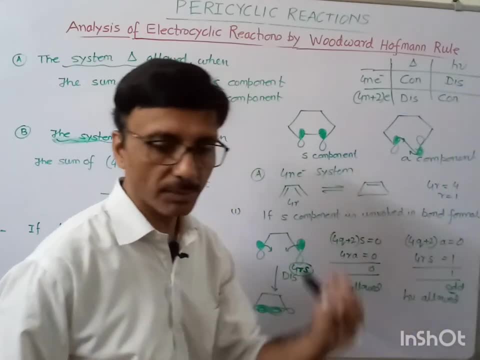 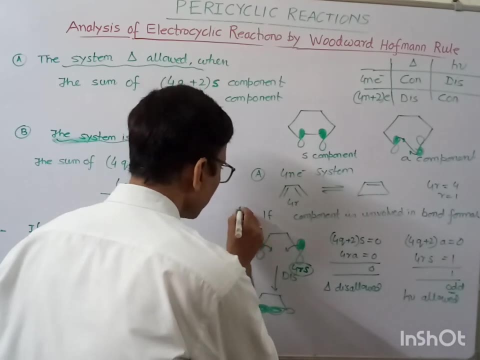 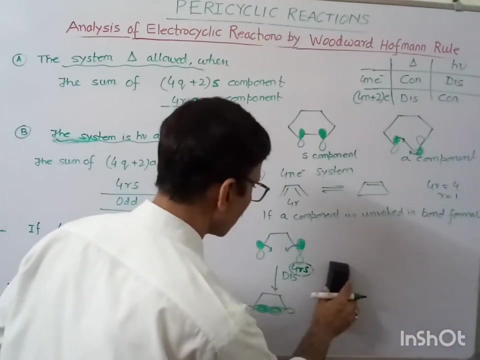 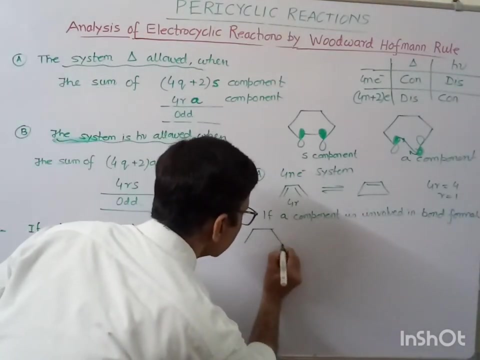 the photochemical condition. this rotation occurs under the photochemical condition. Now if suppose A component is involved in bond formation- second case I will take- when A component is involved in bond formation, then if A component is involved means this is our. A component means when opposite loops are involved in the bond formation. this is 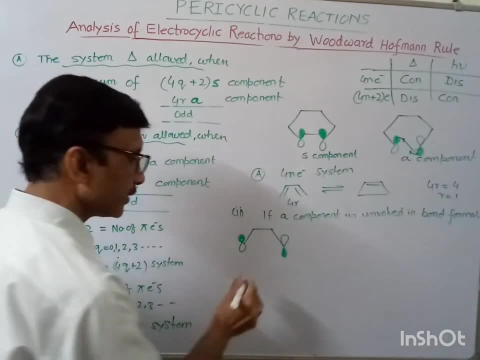 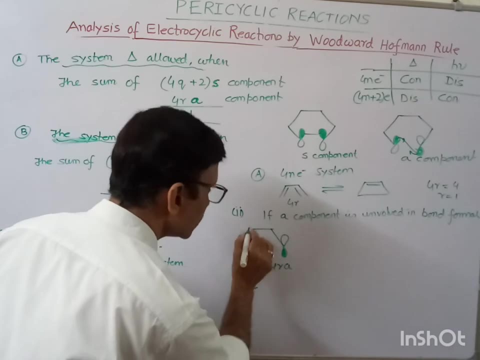 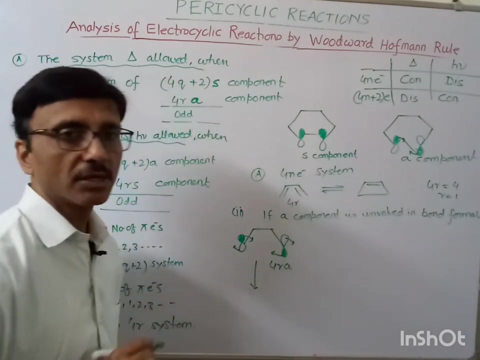 our A component. So what kind of system now it will be. it is 4R component. now they will undergo the bond formation. Bond is only formed. bond is only formed when this will undergo the con rotation, when they will move in a same direction. when they moves in a same direction, then only this bond will. 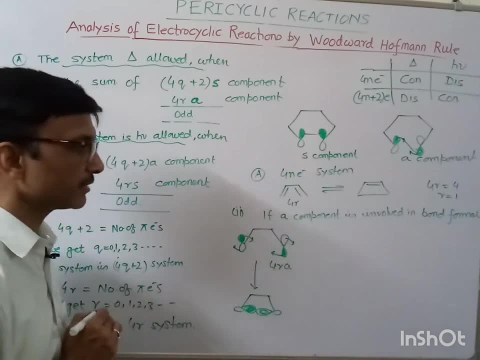 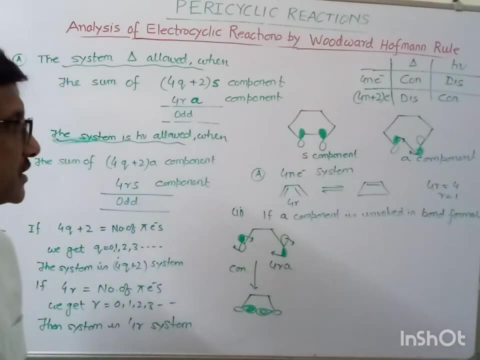 get formed. this bond will get formed when they moves in the same direction. okay, So now let us check this con rotation of orbital is allowed under thermal condition or under the photochemical condition? so we have to check. So first of all, 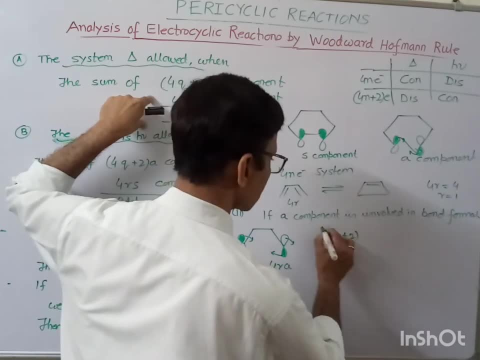 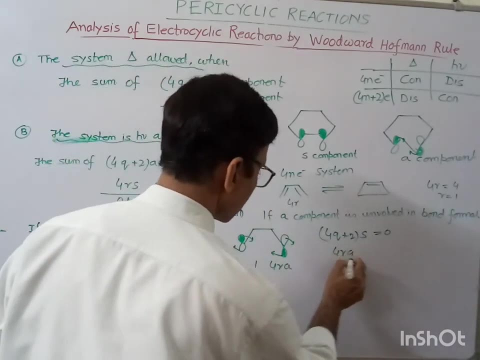 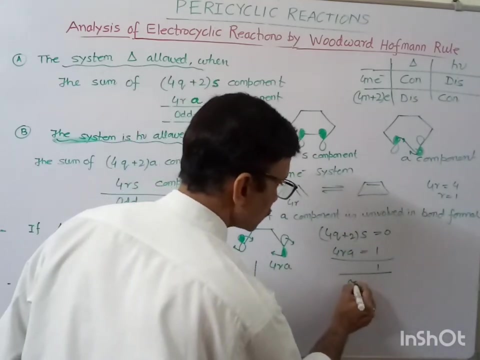 First of all, see this: 4Q plus 2S, this is zero, no doubt, and 4RA, 4R- yes, this is 4RA, so 4RA component is 1, so the sum is coming out to be odd. so if sum out is coming out, 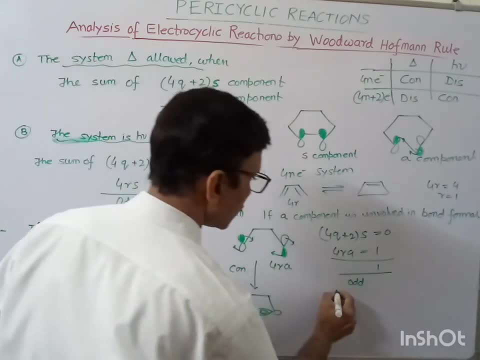 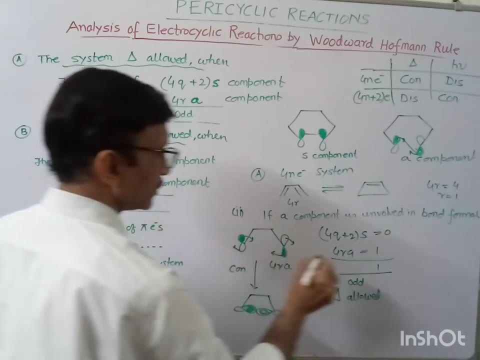 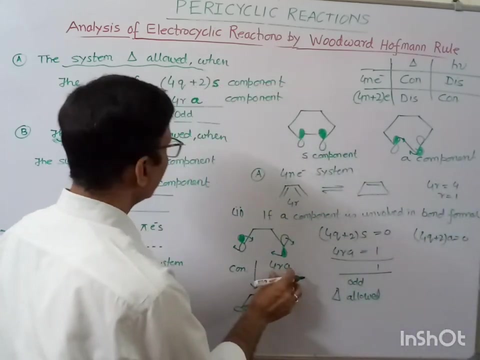 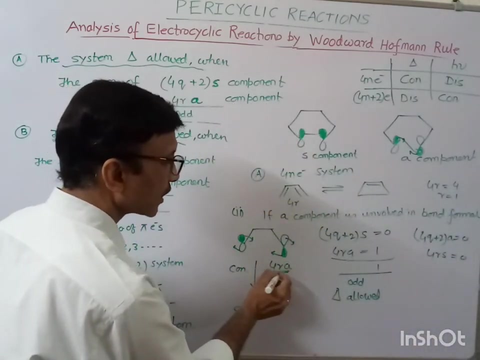 to be odd. it means this is thermally allowed. this is thermally allowed. in a same way, we should check for this one: 4Q plus 2A, this is zero. but and also the 4RS. 4RS is also zero because this is 4RA component. 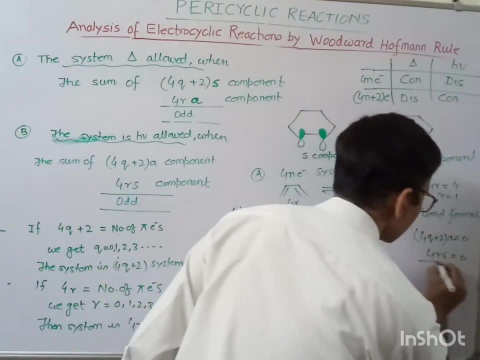 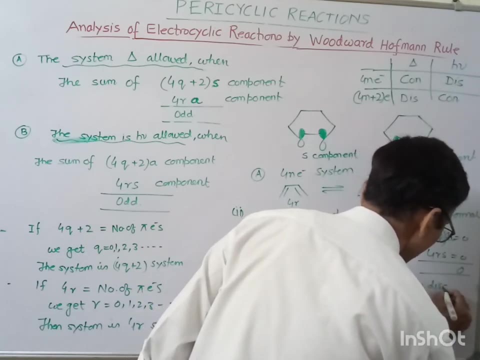 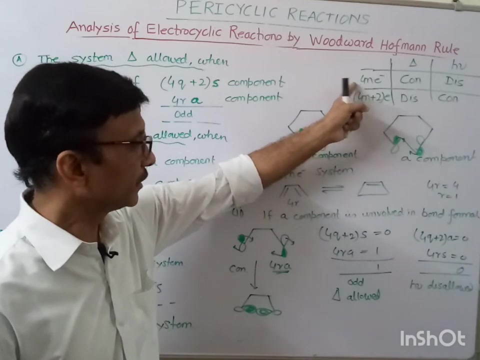 which we have taken over here. so this comes to be overall zero. so it is not odd. so that's why it is photochemical. it is allowed. So we can check the rule For 4N electron system if con rotation is only possible. con rotation is only possible. 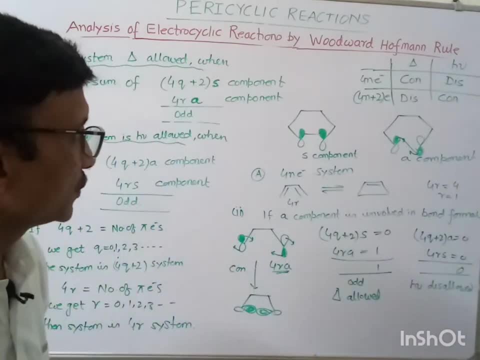 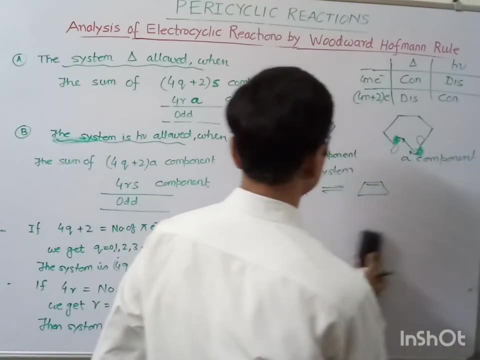 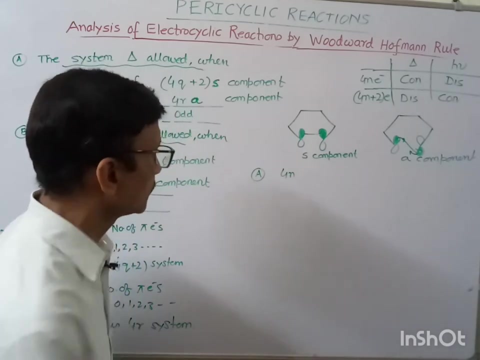 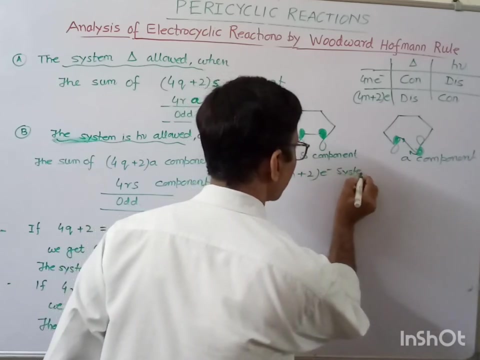 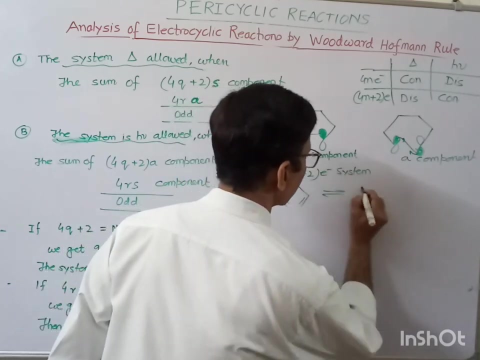 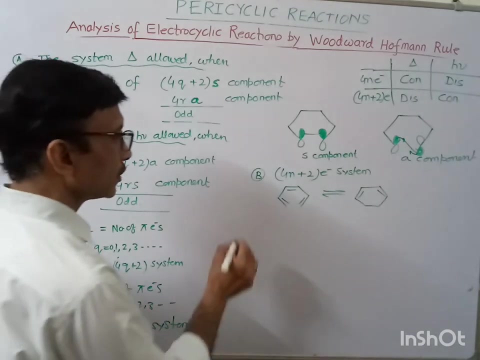 under the thermal condition. okay, So this is for 4N electron system. we may take the 4N plus 2 electron system also. 4N plus 2 electron system, For example, when hexatrine converts up into cyclohexatine clear. so what kind of system? 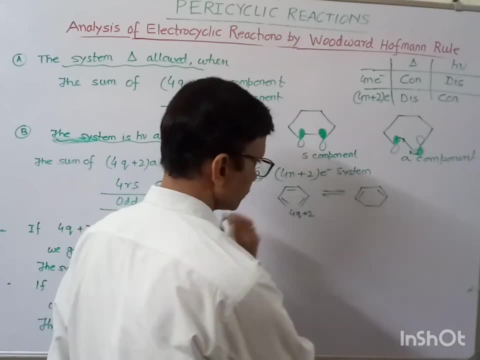 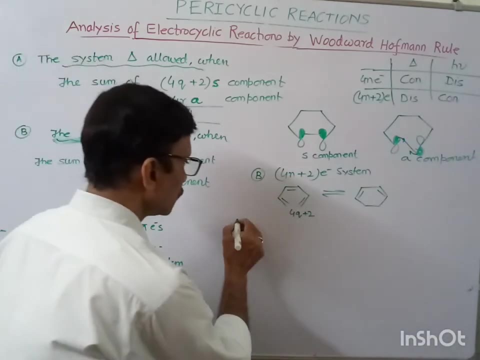 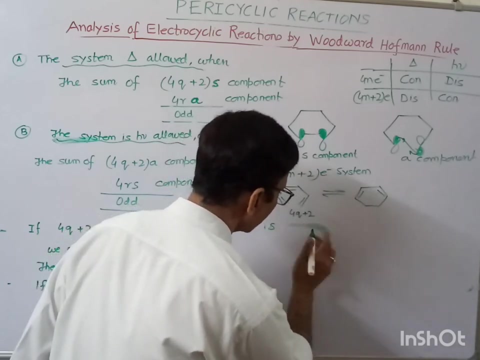 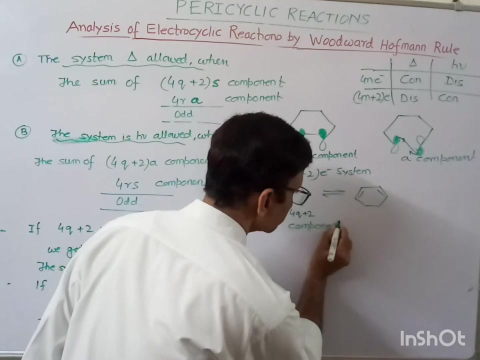 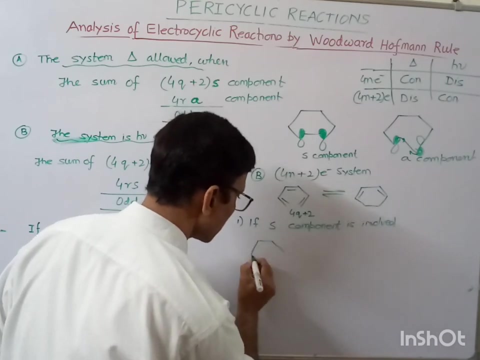 this is. This is our 4Q plus 2 system. now we may take two cases: either 4Q plus 2S or 4Q plus 2A, suppose if S component is involved. if S component is involved means both upper lobe. 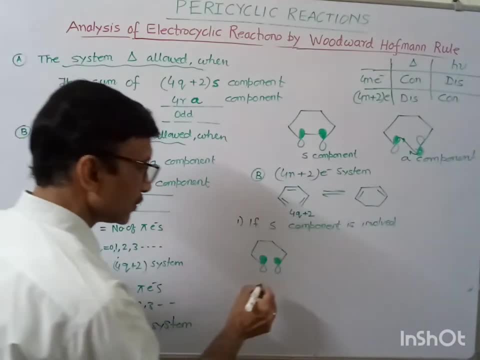 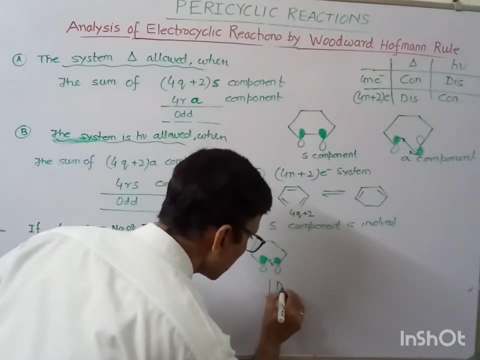 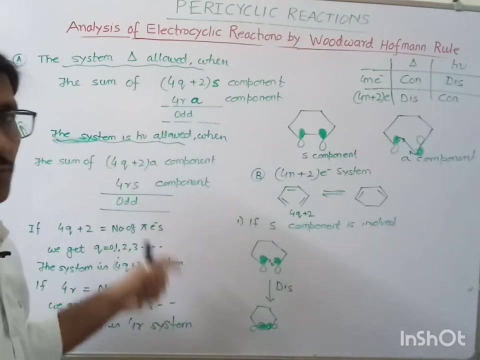 of end orbitals are involved in one form. Okay, So we can take one formation. so the bond will get formed only when they will rotate in a dis-rotatory manner. so then only you will get the bond formation. So now we should check whether this dis-rotation is allowed under thermal condition or photochemical. 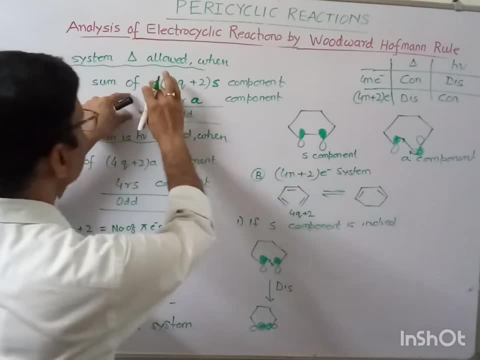 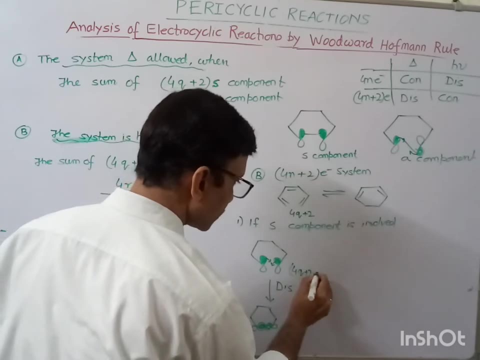 condition. Okay, So under thermal condition we should check the sum of these two components. So what kind of this component it is now? It is 4Q plus 2S component. it is 4Q plus 2S component. 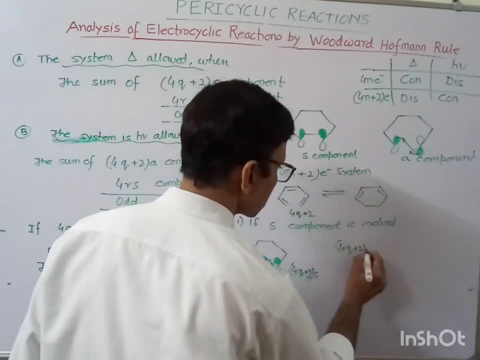 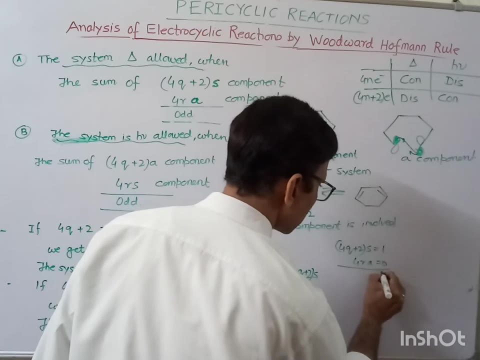 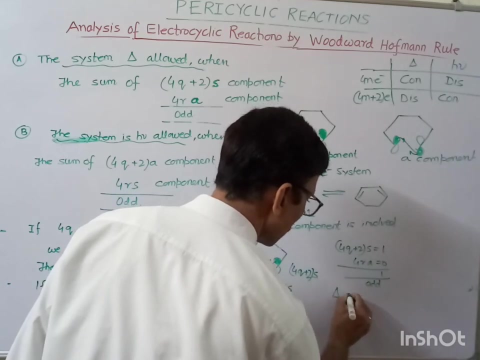 Now this 4Q plus 2S, this is equal to 1. over here, 4RA, this is 0, so it comes out to be 1, and 1 is. this is odd. so if it is odd, it means this is thermally allowed. it is. 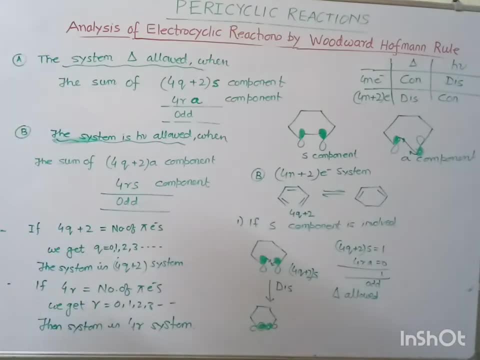 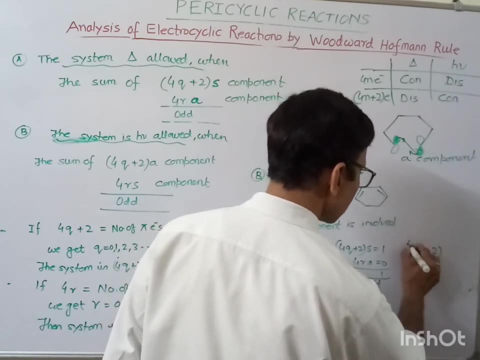 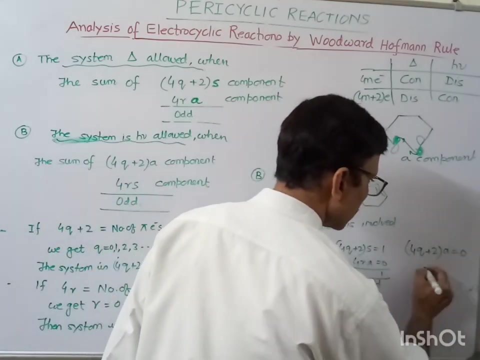 thermally allowed. Okay, Okay, Now we may also check for this photochemical case. so 4Q plus 2S, 2A. this is no doubt this is 4Q plus 2S. that's why 4Q plus 2A is 0, and 4RS is also 0. 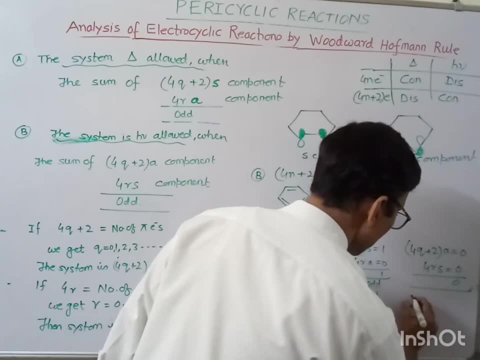 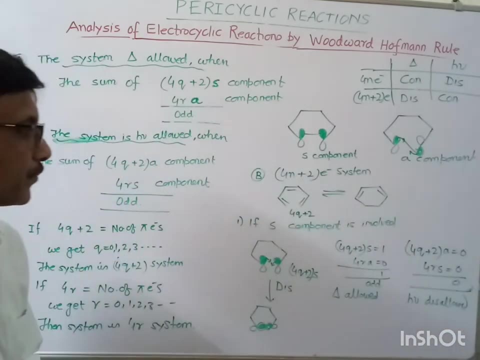 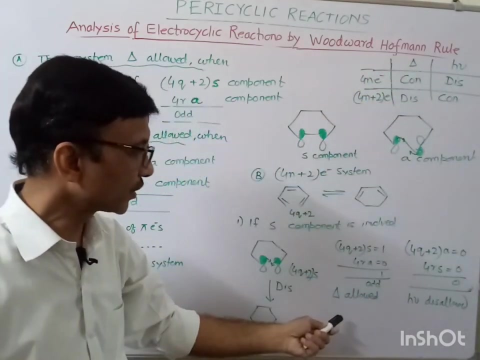 So this comes out to be 0, it is not odd, so that's why it is photochemically disallowed. photochemically disallowed, So what we can see? Okay, So 4N plus 2 electron system. this rotation is only allowed under the thermal condition. 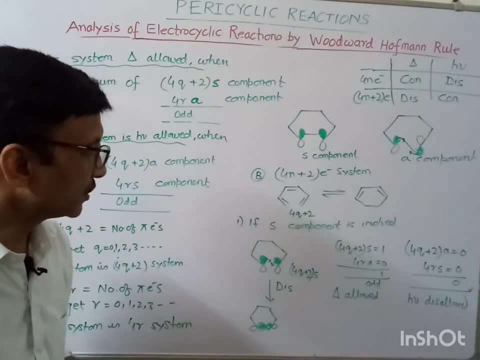 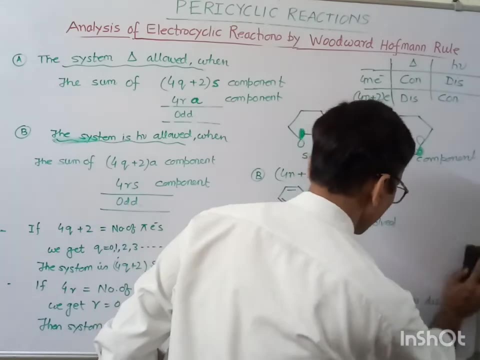 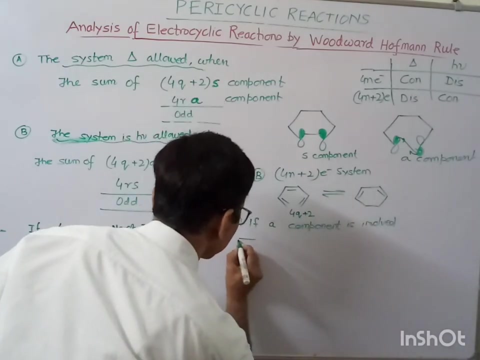 this rotation is only allowed in thermal condition. So in the same way we may check for the A component, we may check for the A component. Let's see A component. What is A component When N orbital in N orbital the opposite, 2N plus 2A, is allowed? 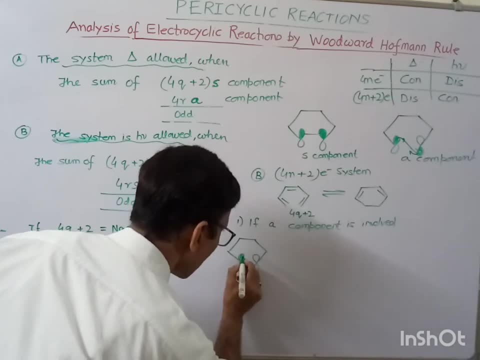 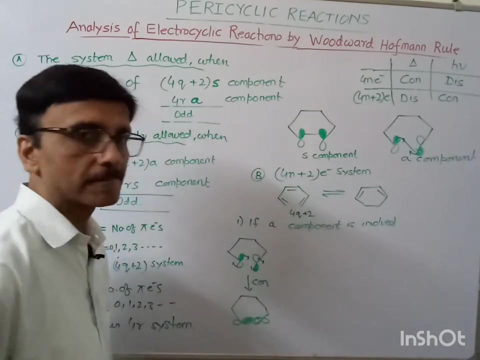 Okay, Okay. So the opposite loops are involved. So this will only form the bond if it undergoes a conrotation. So both moves in a, both orbitals move in a same direction. So conrotation Now, whether this conrotation is allowed under thermal condition or photochemical condition. 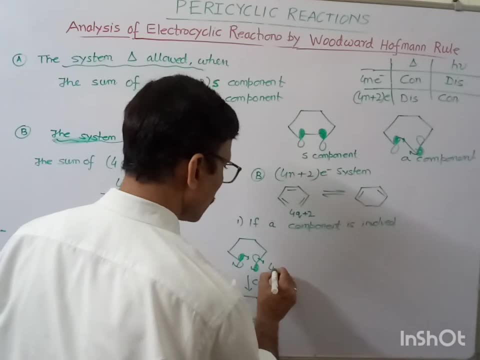 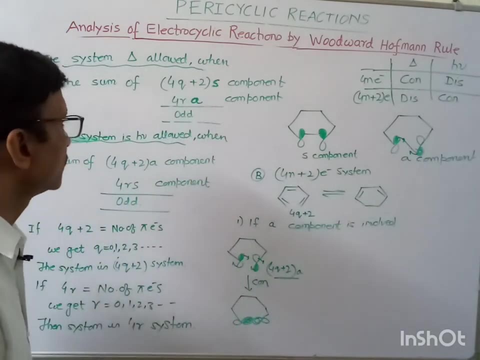 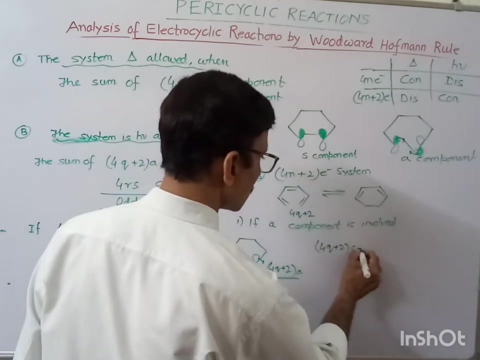 we should check. So let's see. So this is our 4Q plus 2A type of system, because here opposite loops are involved. So 4, whether this is thermally allowed, let's see 4Q plus 2F. this is equal to 0, and 4RA. 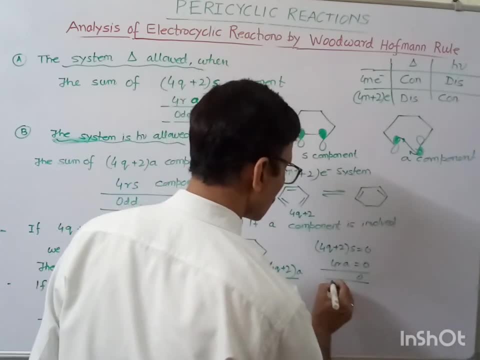 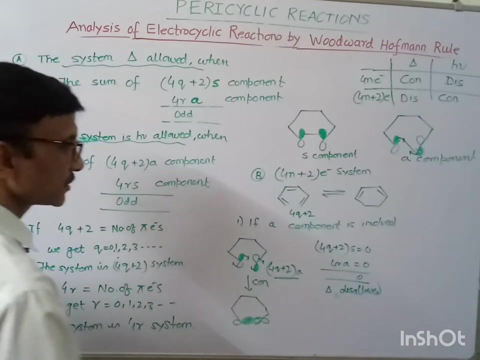 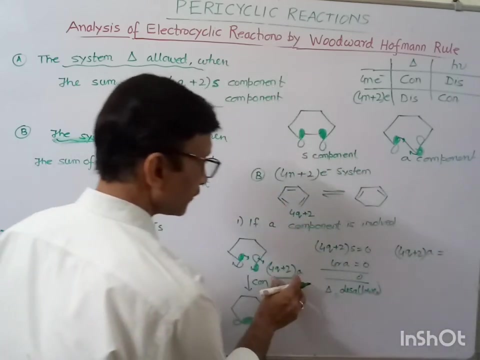 this is also equal to 0,. this doesn't come out to be odd, so it means this is: this is thermally allowed. this is thermally disallowed. This is thermally disallowed. In a same way, let's check for this photochemical case: 4Q plus 2A: this is 1,. this is 1, 1 component. 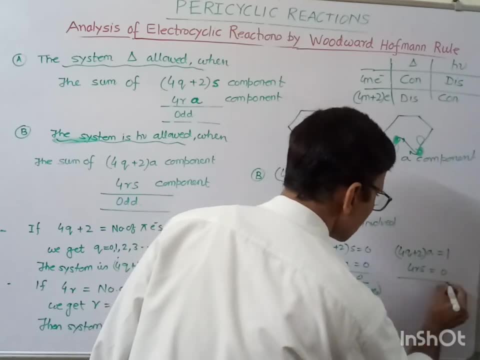 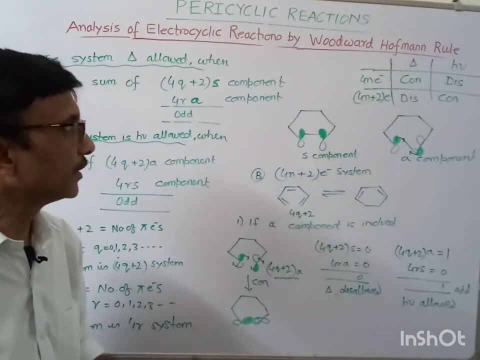 and 4Rs. this is 0, so some comes out to be odd. if some comes out to be odd, it is therm photochemically allowed. Okay, Okay, Okay. So we can see for 4N plus 2 electron system. so for 4N plus 2 electron system, under when? 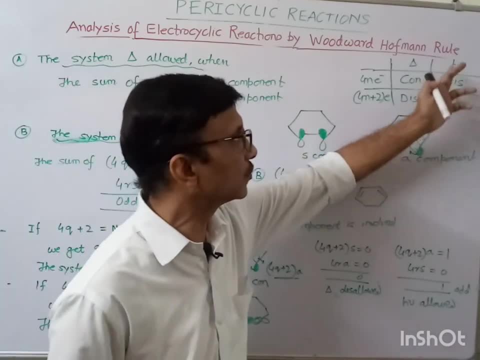 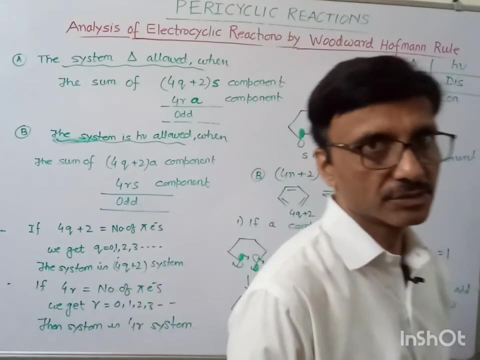 conrotation. the conrotation is only allowed under the photochemical condition. So this is about the electrocyclic, this is the Woodward-Hoffmann rule. So now we have analyzed the this Woodward, this rule. electrocyclic rule for invariant.